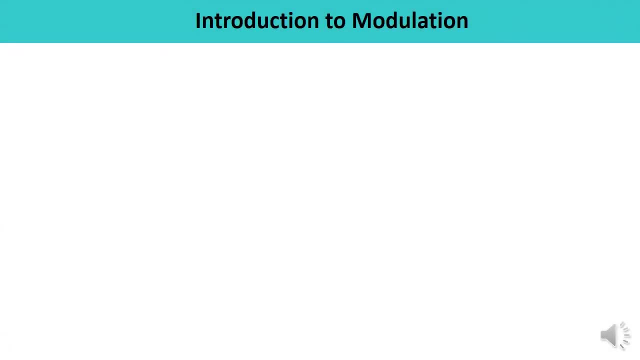 To start with, let us revise: what is modulation, what is communication? just to give you a review- I know you are already aware it, but just to have a look on the communication and modulation: See communication. it is a process of transferring information from one place to the another place. 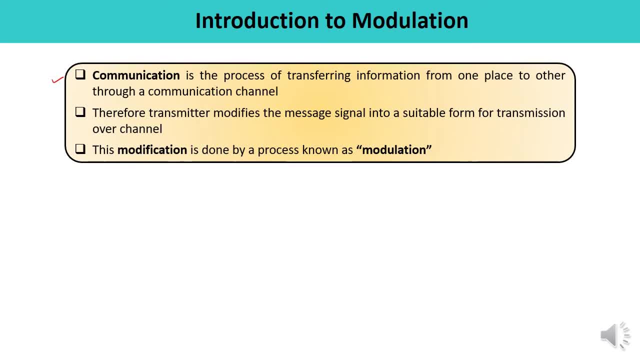 via a communication channel. Like I am speaking something, you are listening something. So this is what a communication It means. for communication, one transmitter modifies the message signal which is to be transmitted and that message signal must be modified into some suitable form which is suitable for the transmission over the channel. 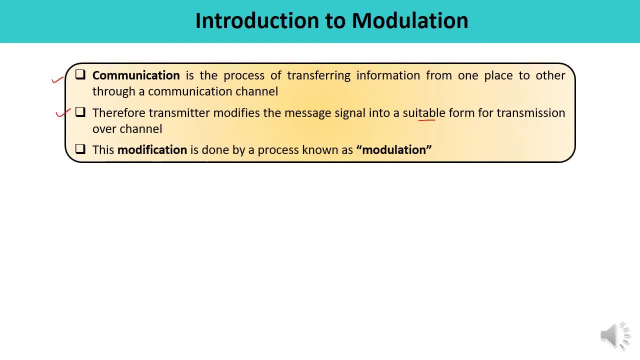 And this modification. this process is known as a modulation. So how you can define the modulation? Modulation is defined as a process by which some of the characteristics of the carrier signal is vary According with the instantaneous value of the modulating signal. right? 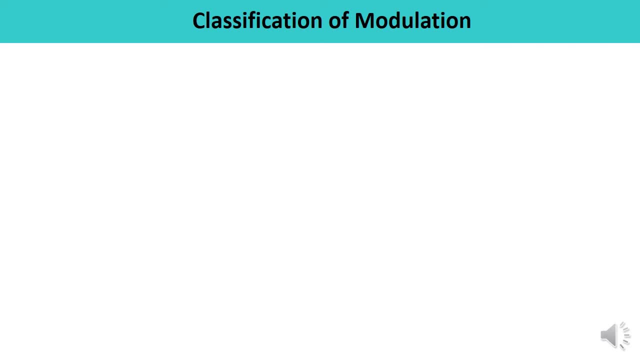 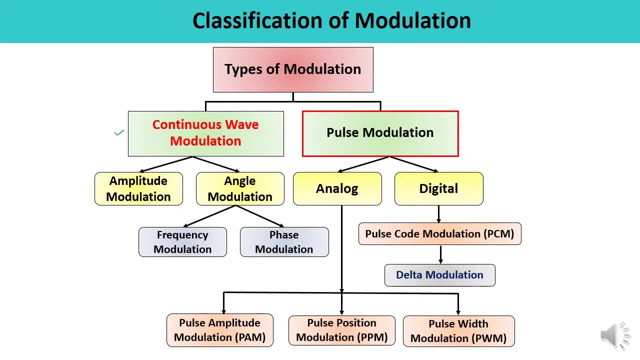 Classification of modulation. So first let us understand that initially it is categorized into two category. First is the continuous wave modulation, So in case of continuous wave modulation the carrier is continuous signal. Second is pulse modulation, and here carrier is of pulse strain. 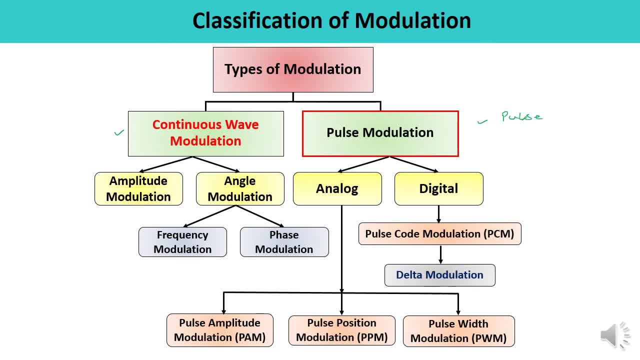 So you must remember that what is pulse modulation Here? carrier is different. In this video I will be talking about the pulse modulation, But you must remember that continuous wave modulation is of two types, which is amplitude modulation and angle modulation. Angle modulation is also of two types. 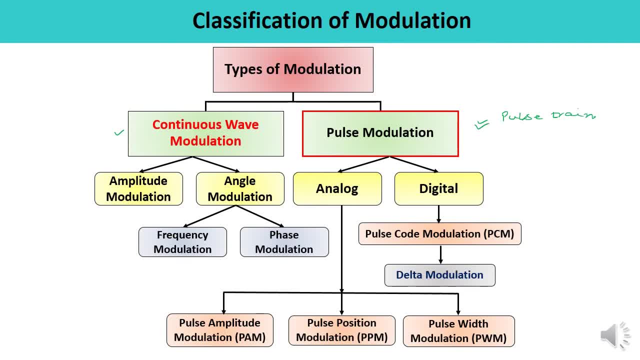 which is frequency modulation and phase modulation, And in the previous videos I have talked about the continuous wave modulation. So let us focus on the pulse modulation. So you must remember that in pulse modulation method the carrier is no longer a continuous signal, but it consists of a pulse. 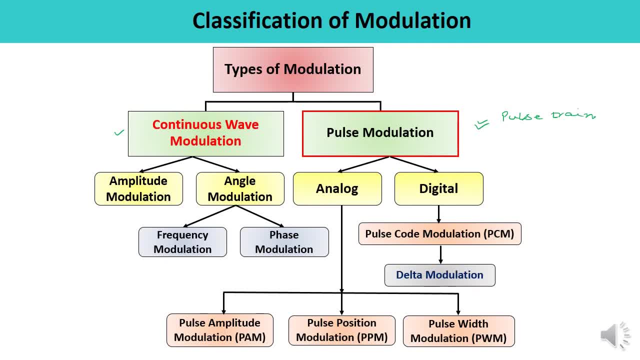 strain and some of the parameter of which is varied according to the instantaneous value of the modulating signal, means parameters of the pulse strain, which is the carrier signal That is being varied. it so accordingly, there are three types of analog pulse modulation. one is pulse amplitude modulation. 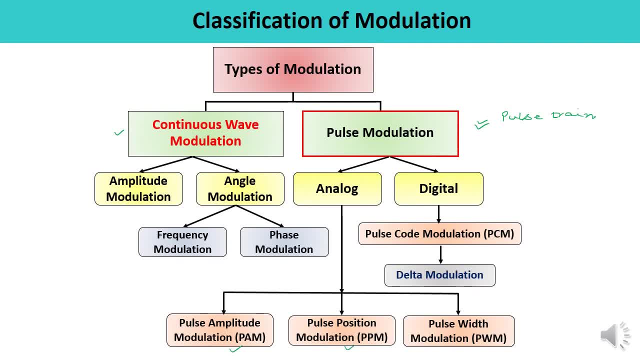 where amplitude varies. second is pulse position modulation, where position varies, and third is the pulse width modulation. so this pulse position modulation, which is ppm, pulse width modulation, which is pwm, these two are actually pulse time modulation. so, pulse position and pulse width, these are the types of pulse time modulation where the timing of pulses, of carrier pulse. 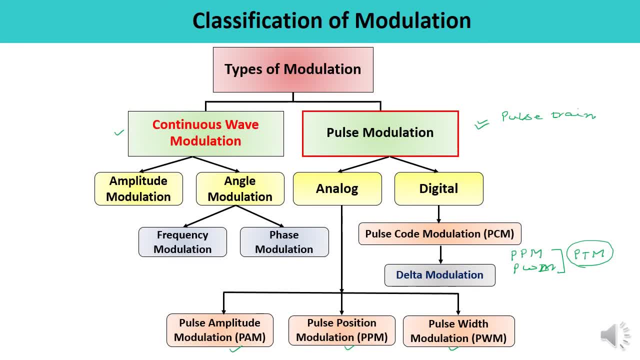 strain is actually varied right. second category of pulse modulation is digital, where pulse code modulation is a technique and delta modulation is also a digital technique. so we are going to talk about in coming video lectures in detail about the pulse modulation. you must remember that pam, pwm, ppm, these are the analog pulse modulation because 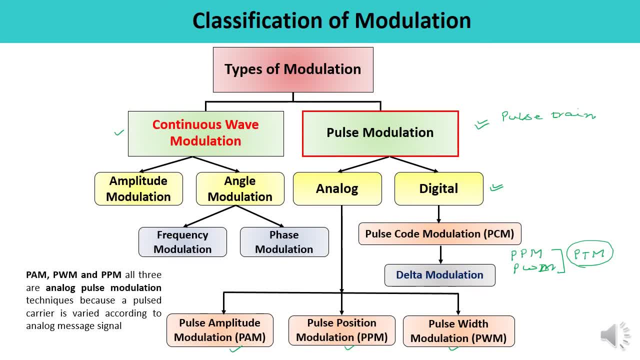 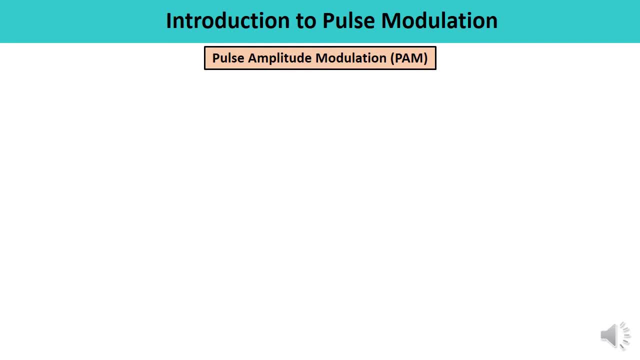 pulsed carrier is varied according to the instantaneous value of the message signal. now, what is pulse amplitude modulation? as i have already told you that in pulse amplitude modulation the amplitude of pulsed carrier is varied according to the amplitude of analog modulating signal means, according to its instantaneous value. we can draw the waveform as: 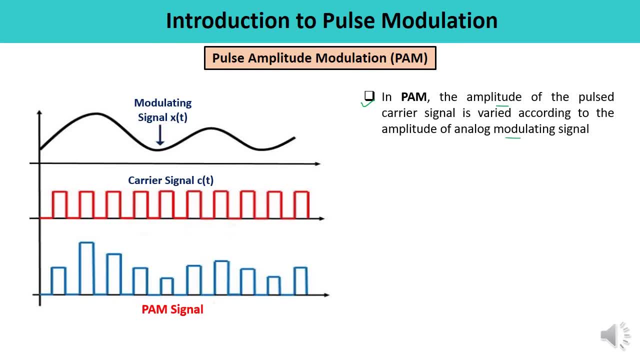 well, you can see: first we have drawn a modulating signal, which is the xt, then a carrier signal. here the carrier signal is a pulse strain. now you can see the third one, it is the pam signal, pulse amplitude modulated signal, and you can see how the carrier is varying according to the amplitude of 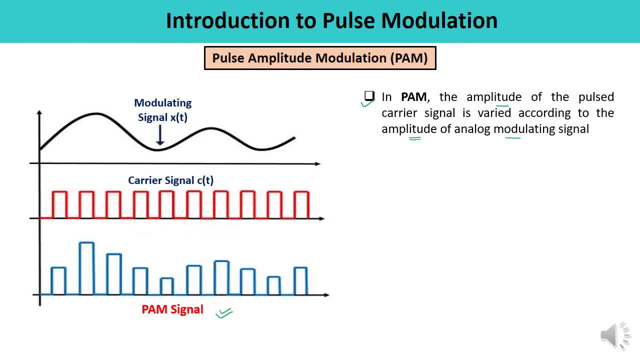 the modulating signal. so accordingly you are. you can see over here how amplitude is varying according to the modulating signal. at this point amplitude is high, so this kind of pulse is being drawn. at this particular point, you can see, amplitude is less, so this type of pulse is being drawn. 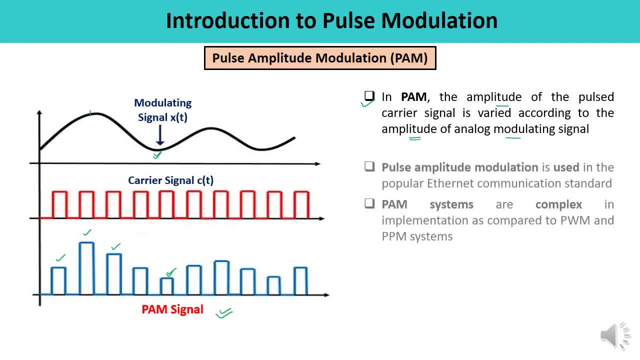 so this is the pulse amplitude modulation signal: pulse amplitude modulation. it is commonly used and it has a popular application in ethernet communication. pam systems are very complex and their implementation means the implementation of pam system. this is complex in comparison to the ppm and pwm, so in the coming video lectures we 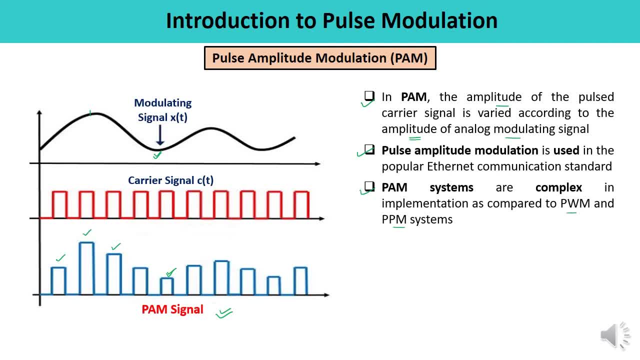 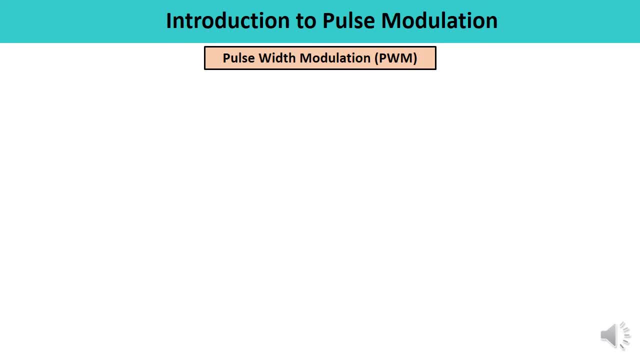 are also talking about the modulation and demodulation. second is the pulse variation and the pulse width modulation. as i have already told you that, it is a type of pulse time modulation. so in case of pulse width modulation, the width of the pulse of carrier wave is varying according to. 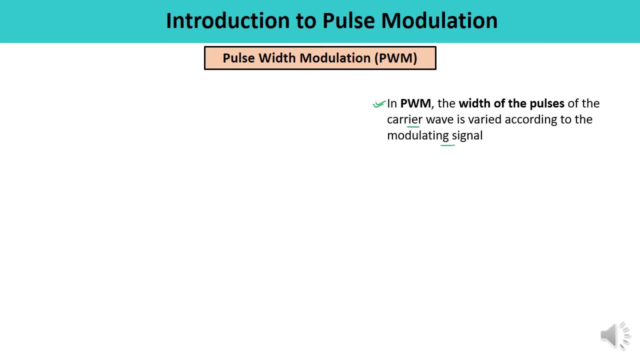 the modulating signal. so i hope now, with the help of the modulating signal and the carrier signal, you can draw the pulse width modulated signal, pwm signal: see first is the modulating signal, second is the pulse width modulation signal and as i have told you that here the width of the pulse changes, 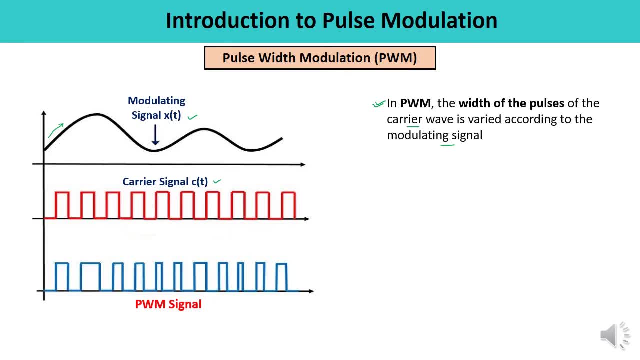 so you can see as the modulating signal varies its amplitude. you can see here the variation. here the value is less. at this particular point the value is high. at this point you can see how width of pulse is being varied accordingly. when it is being decreasing, the width is being decreased. 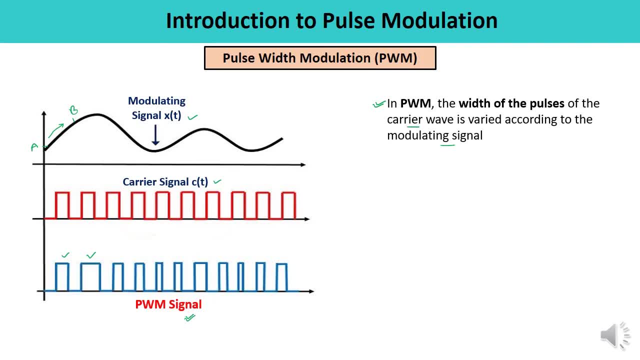 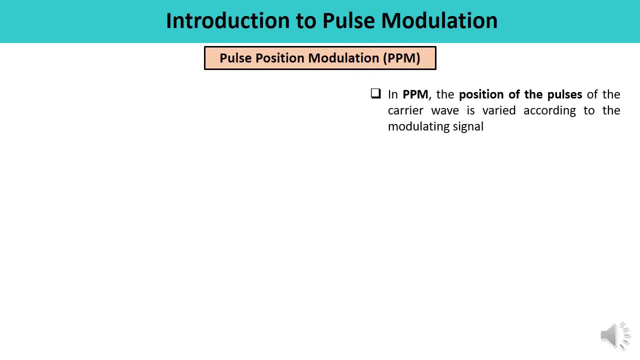 again. so in this way you can draw the width of pulse width modulated signal. next is the pulse position modulation in ppm. the position of pulses of carrier wave is varied according to the modulating signal. so here position of pulse is varied and this is also a type of pulse time modulation, which is ppm. you can see here our 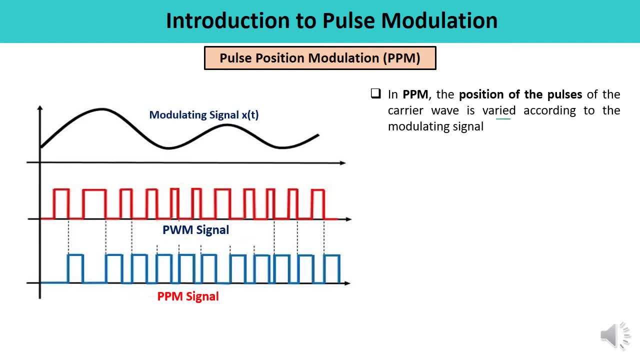 modulating signal is being shown: pulse width modulation signal, pwm, and accordingly ppm signal, this particular case. so here some of the important point. you must remember that the position of pulses changes according to the reference pulses. and what is reference pulse? reference pulses are nothing but the pwm pulses. so first you draw the pwm pulses, then according to the falling edge of 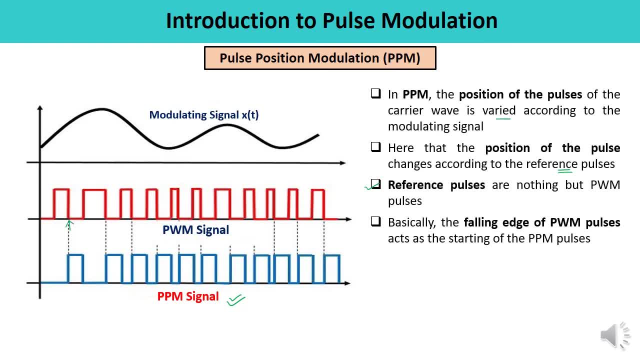 pwm pulse. see, this is the falling edge of pwm pulse. this is the falling edge. this is the falling edge following edge of pwm pulses. it acts as the starting point of ppm pulse. you can see, this is the starting point of pp. next falling edge will be the starting point of the next ppm pulse. next, 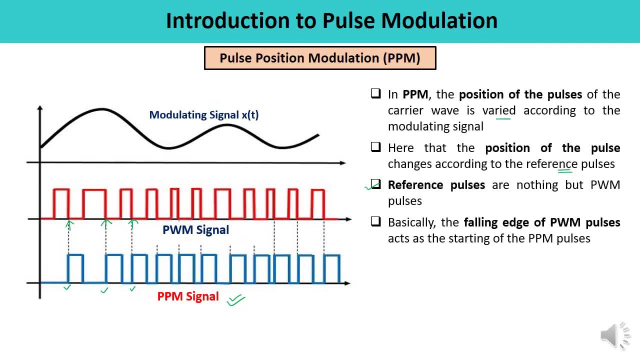 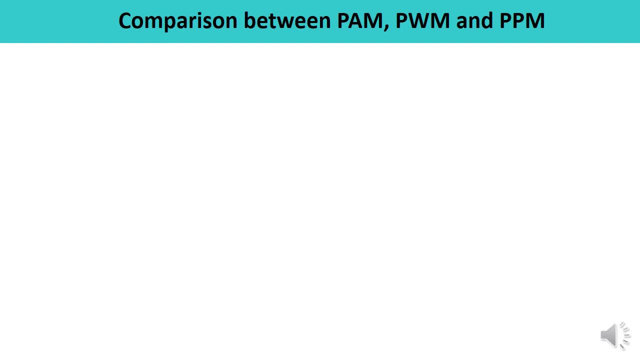 falling point will be the starting point of next ppm pulse. so accordingly it couldn't can be drawn. so i hope now ppm is also clear to you. now let us talk about the comparison between the palm pwm. ppm and this comparison can be done on the basis of the certain parameters, certain 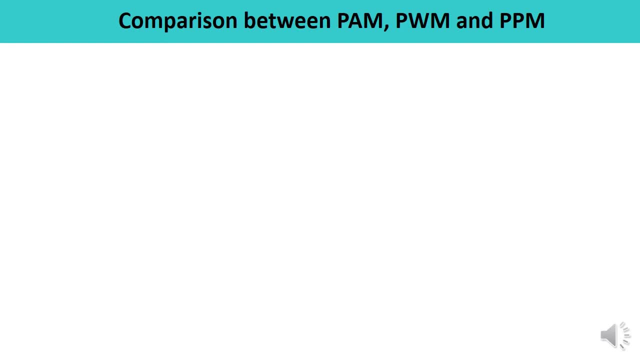 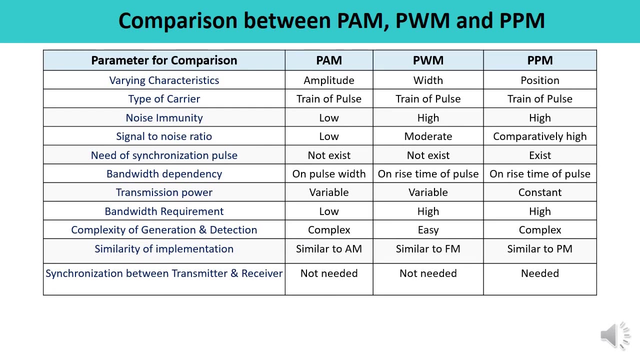 like identified characteristics and i have over listed out over here some of the parameters for the comparison and accordingly, how this palm, ppm and pwm shows their behavior. first, if we talk about the varying characteristic, so the varying characteristic in palm is amplitude, in case of ppm it's a position type of carrier. in all the three cases are train of pulses, noise, immunity. 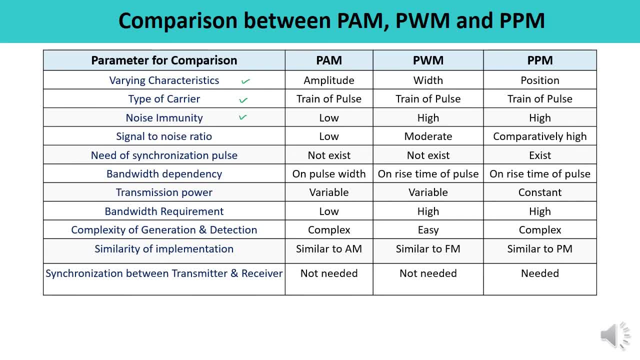 it is low in the case of palm, but it is high in case of ppm and pwm signal to noise ratio is low in case of palm. noise immunity is also less, but it is moderate in case of pwm, but it is high, relatively high, in case of ppm. 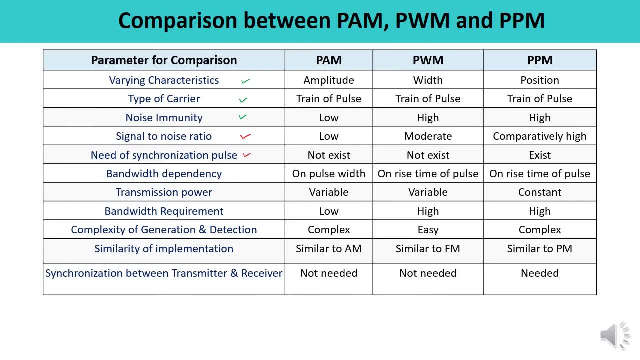 noise to synchronization pulse. it does not exist in palm pwm, but noise to synchronization pulse exists in case of the ppm bandwidth dependency if we talk about, then in case of palm it depends upon pulse width, in case of pwm it depends upon the rise time of pulse, while in case of ppm it also. 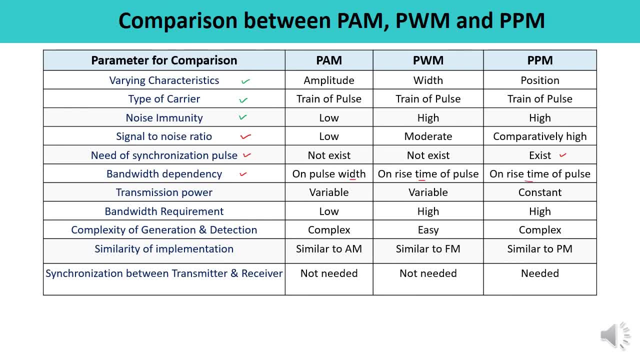 depends upon the rise. time of pulse. transmitted power is variable in palm and pwm, while it is constant in case of ppm. you can compare these three on the basis of the bandwidth requirement. also, bandwidth requirement is low in case of palm, while it is high in case of pulse time modulation. 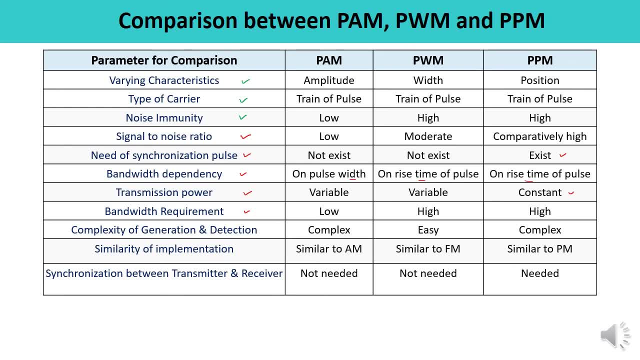 which is pwm and ppm. complexity of generation and detection. palm signals are relatively complex for generation and detection. pwm is easy, but ppm is also complex if we talk about the similarity of operation, how this palm, ppm and pwm works. if you would like to recall in which particular manner means to which particular operation it resembles, then palm is. 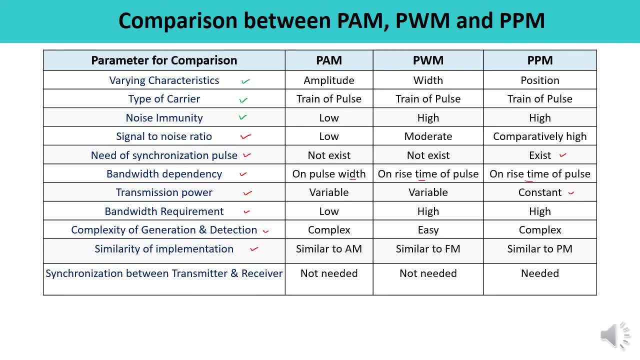 like a similar to amplitude range, but ppm is similar to amplitude range and ppm is similar to amplitude range modulation. pwm is like similar to frequency modulation and ppm is similar to the phase modulation. next and last parameter for the comparison is the synchronization between transmitter and receiver. so synchronization is not required in case of pam. it is not required. 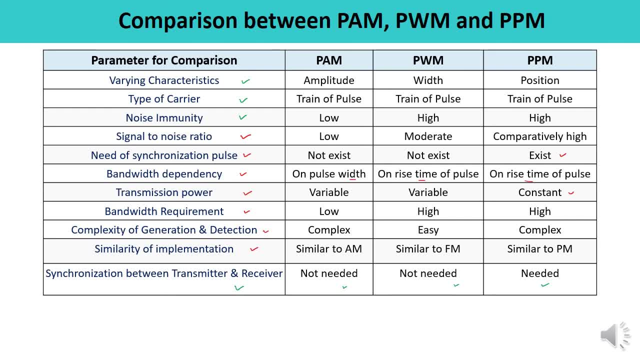 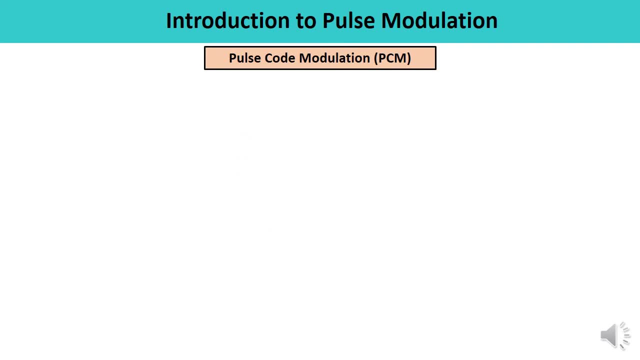 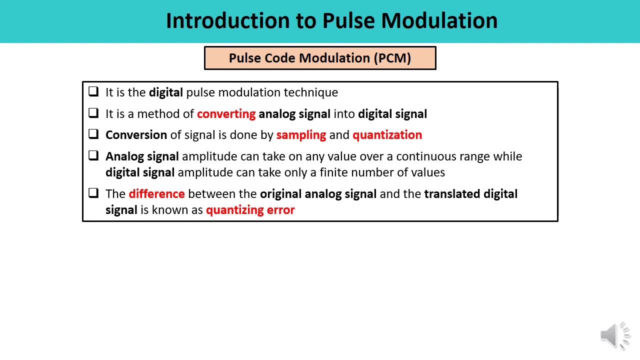 in case of pwm, but it is required in case of pulse position modulation. so these are certain parameters upon which the comparison between pam, pwm and ppm has been done. next, let us talk about the pulse code modulation, which is the another category of pulse modulation. pulse code modulation, it is a digital pulse modulation technique because initially we have 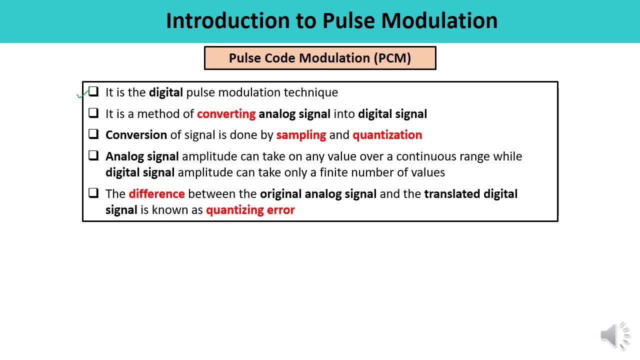 seen that there are two categories in the pulse modulation. one is analog pulse modulation. second is digital pulse modulation. in analog pulse modulation we have studied three types of modulations, which is pam, pwm and ppm. so this is the digital pulse modulation technique and it is a method of converting analog signals. 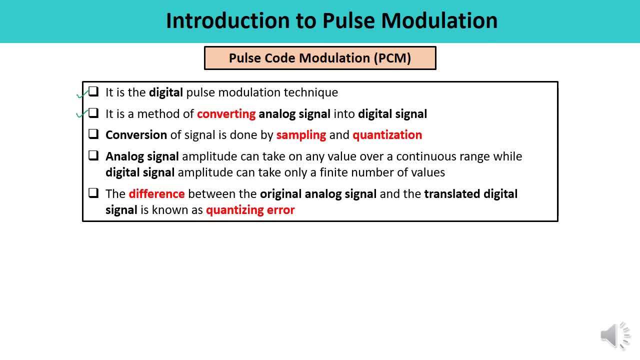 into the digital signals. so via pcm, analog signals can be converted into the digital signals and for this particular conversion, the process which is to be performed. that process includes sampling and quantization. so the conversion includes sampling and quantization. if we talk about the analog signal amplitude, it can take any value on a continuous range, while digital signal amplitude can take